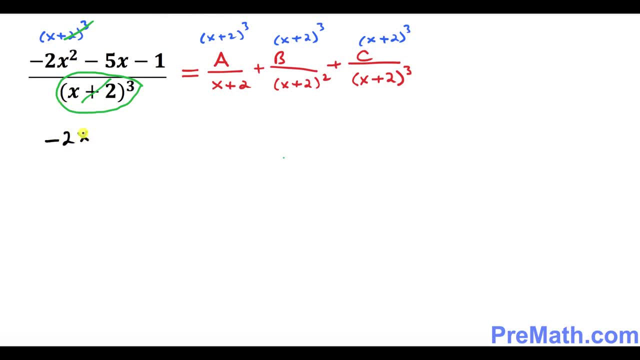 we're going to get on the left hand side, negative 2x power 2 minus 5x minus 1 equals to one of these factor cancels out. So we got a times x plus 2, square plus b, times x plus 2, as you can see, and finally, you can see this: 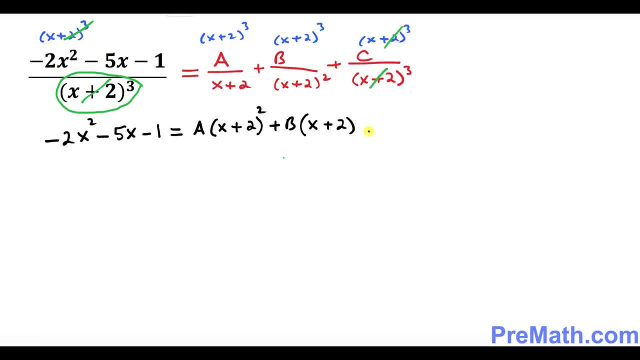 whole thing cancel with this one. so we got plus c. i want to call this equation number one, just keep in your mind. so now we want to find the value of a, b and c. so we will be using this simple trick. what we did is at the bottom, you see, at the denominator, we have linear factor x plus 2. i. 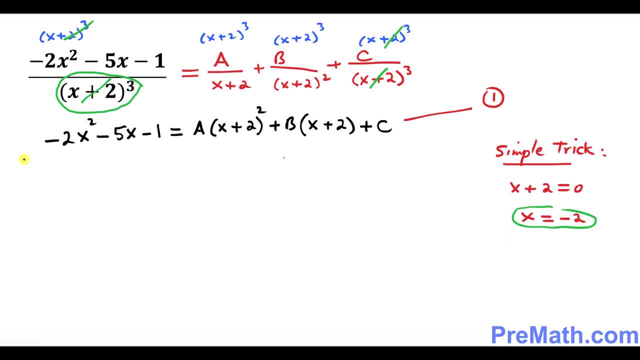 just set that thing equal to 0. x turns out to be negative 2. so that's what i'm going to do. i'm going to say, at x equal to negative 2, what's going to happen? let's go ahead and plug it in in this equation. 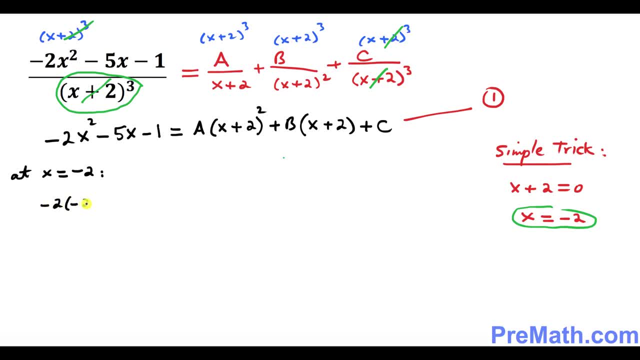 number one. so negative 2 times negative 2 square minus 5 times negative 2 minus 1 equals to do. you see this thing over here a time. negative 2 plus 2 is going to give you 0: 0 square is 0, of course, plus b times negative 2 plus 2 is again 0 plus c. 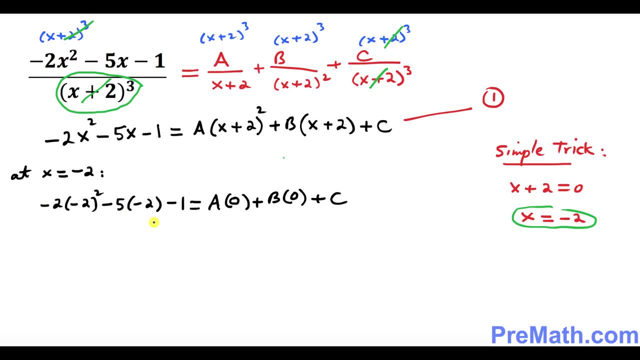 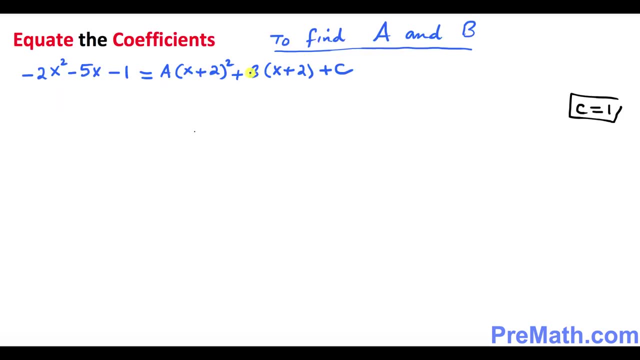 so once you simplify this thing over here on the left hand side, that's going to give you 1 on this side. so, and this is 0, this is 0, so c turns out to be 1. so the next thing we want to find a and b. 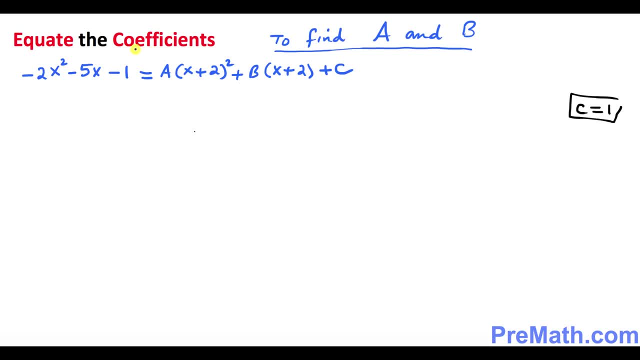 and we will be using this method. it is called equate the coefficients or simply compare the coefficients on the both side. let's see how things go. let me show you now. so we're going to put down a times x plus 2 squared. you just multiply twice. the square is going to be: 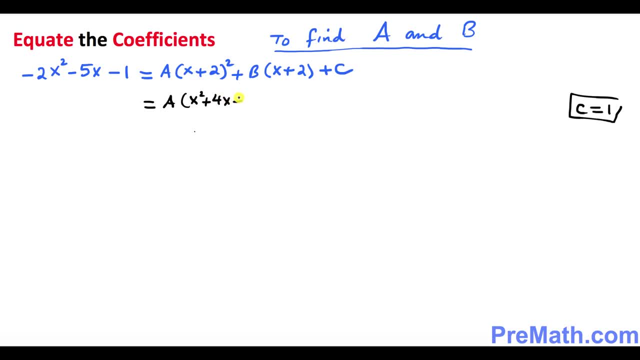 x squared plus 4, x plus 4. and then i want you to just simply distribute this thing. that's going to be plus b, x plus 2, b plus c, or simply we're going to distribute over here as well. so that's going to be a x squared plus 4, a x plus 4, a plus b, x plus 2, b plus c over here. so let's go ahead and look at: 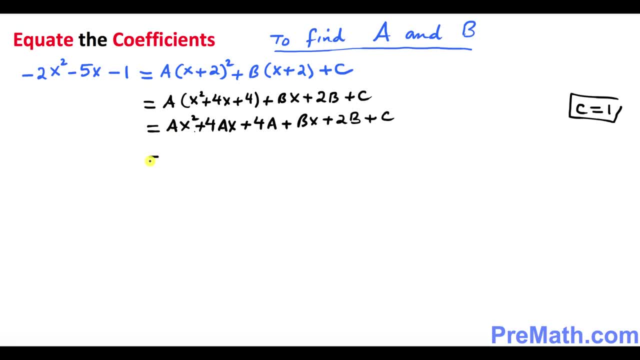 what we got. so we can write: see, only there's x square part. so I'm going to write down a x squared plus. how about for x parts? this is x, this is x. so that's going to make 4 a plus b times x plus what is going to be the constant terms: 4 a plus 2 b and then plus c. 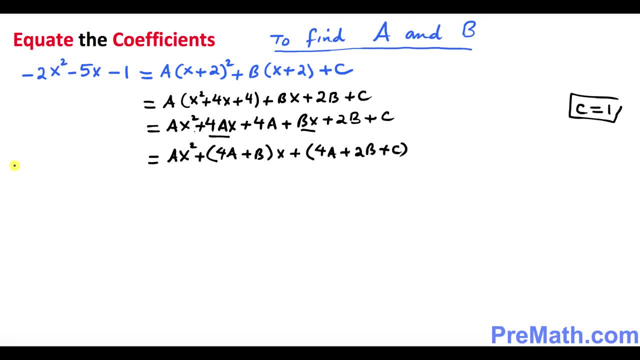 on the right hand side and on the left hand side is simply negative. 2x squared minus 5x minus 1. so now we're going to compare these terms on both sides, so let's focus on the square coefficients. on the left hand side, this is a negative. 2 equals 2. on the right hand side, we just simply: 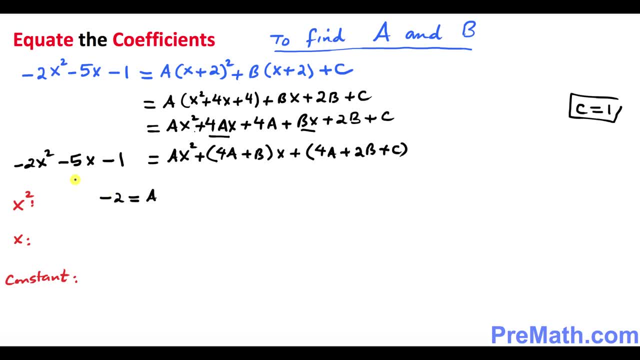 got a, isn't it? so for x is going to be: for x variable, the coefficient is negative. 5 on this side equals to 4 a plus b, and for the constant is going to be a negative 1 equals to 4 a plus 2 b plus c.